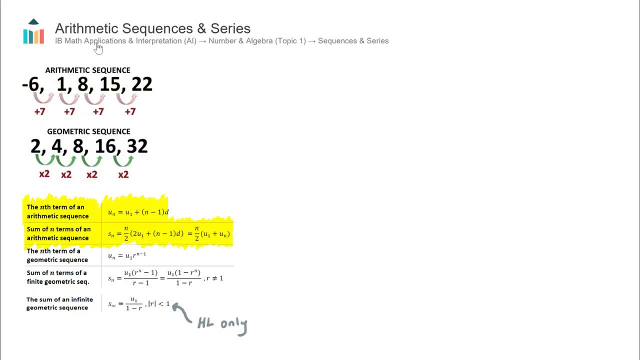 This video covers arithmetic sequences and series, an important concept in IB Maths AI found in Topic 1, Number and Algebra. 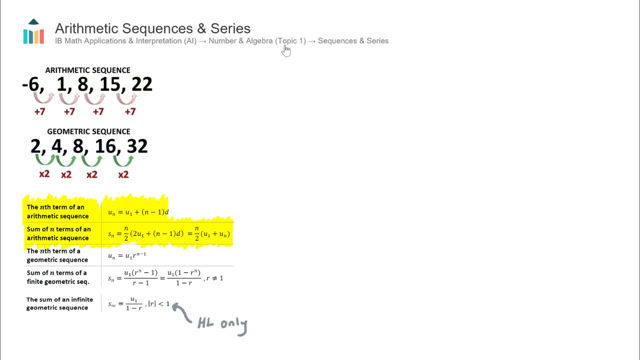 Now, arithmetic sequences and series is one of the two types of sequences that you'll encounter. You'll encounter either arithmetic or geometric, and the difference between the two is that arithmetic goes up by a common difference, or up or down, sorry. So, for example, this sequence of numbers here is going up by a common difference, or addition, or by 7. It can also be subtraction as well. Whereas geometric sequences go up by a common ratio, or a multiplier, as you can see here, the multiplication of 2. So in this video we're going to be focusing on this top sequence of numbers, arithmetic sequences. Okay, so let's talk about this sequence here. I'll just write it out on the right-hand side. So we have a negative 6, 1, 8, 15, 22, and let's assume that this sequence goes on. 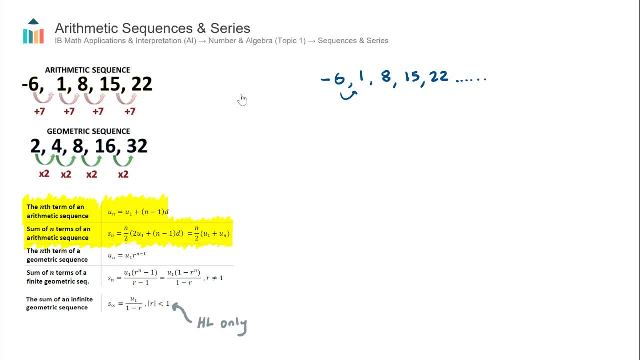 Now, these numbers are going up by an addition of 7, so plus 7 each time. 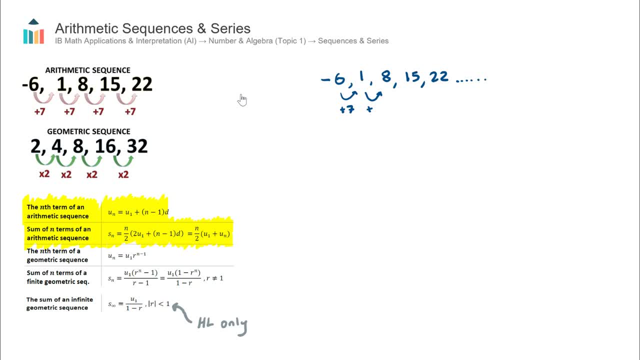 And we call this addition the common difference. So in this sequence here, my common difference, which we call d, is equal to 7. 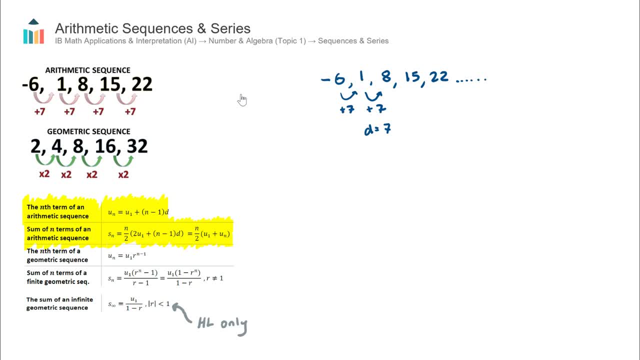 Now, a little bit more terminology. The term numbers we identify with a letter u. So the first term, this negative 6, would be u1. The second term would be u2. The third term, u3, and so on. 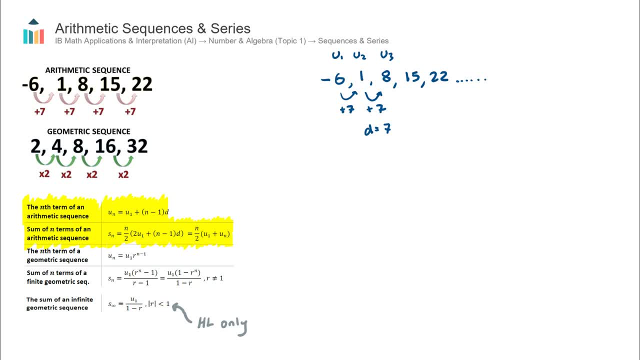 Now let's look at another example of an arithmetic sequence. 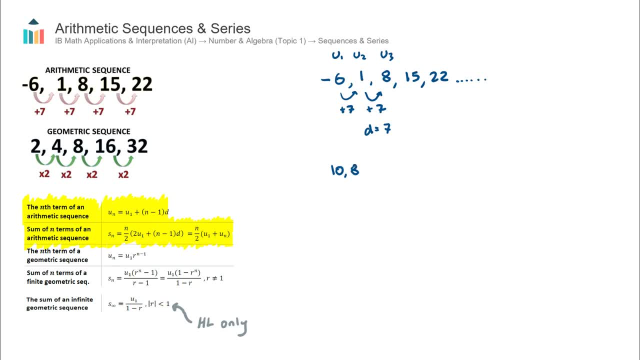 Let's say, let's go 10, 8, 6, 4, dot, dot, dot, dot. 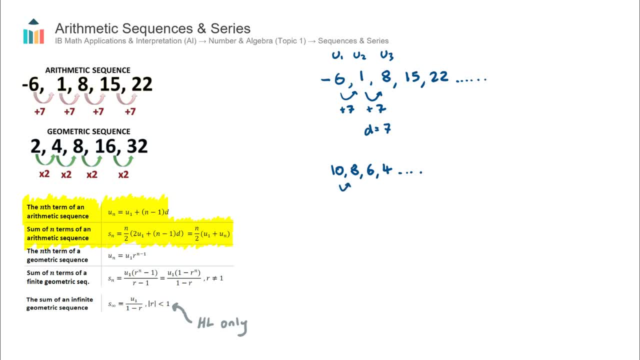 So this is similar, but different in that the common difference is a negative number. So we're subtracting 2 every time. But still, same idea. Here, our common difference is negative 2. 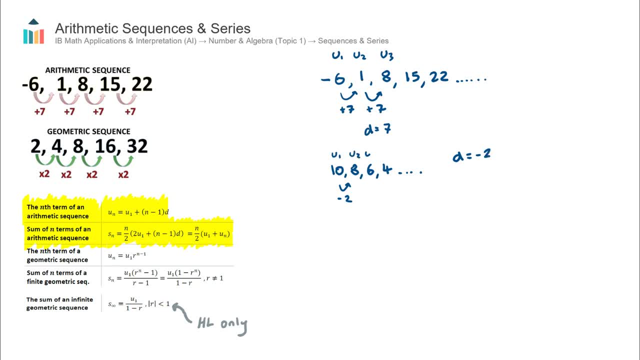 And again, we would call this the first term, the second term, the third term, and so on and so on. 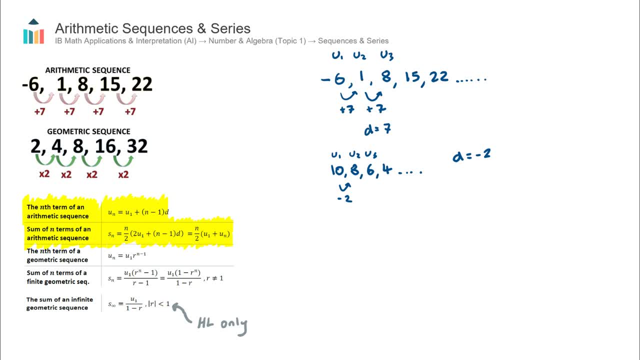 Now, in your formula booklet, you are given a number of formulas related to sequence and series. So you can see there are five here. The top two are related to arithmetic sequences. So we're going to talk about these two in this video. 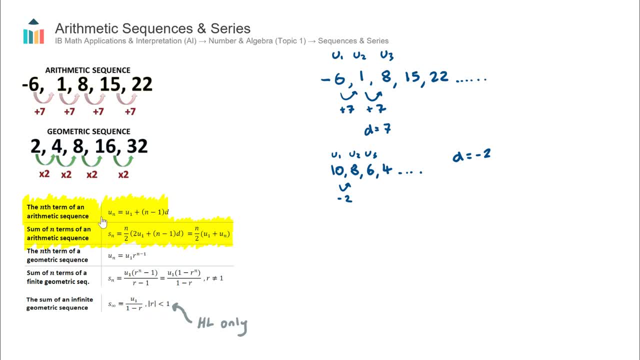 So the first one is very useful to find a particular term in the sequence. So for example, I'll use this example here. I know the first, second, third, fourth, and fifth term. But what if I was to ask you, what's the 15th term, let's say? Now you could start adding 7 each time, but that's quite time-consuming and quite sort of mentally challenging after a while, particularly if I asked you, say, the thousandth term. 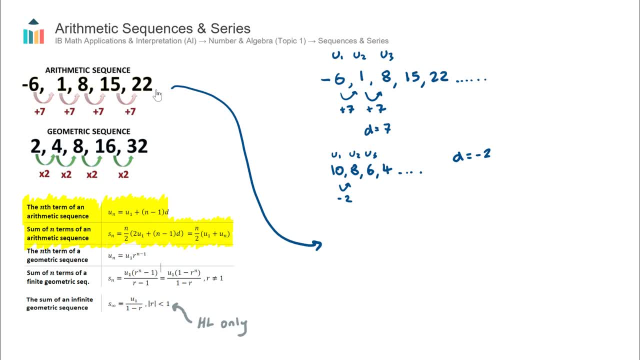 So we need a quick way to find some sort of term in the future. So let's just walk through that now. 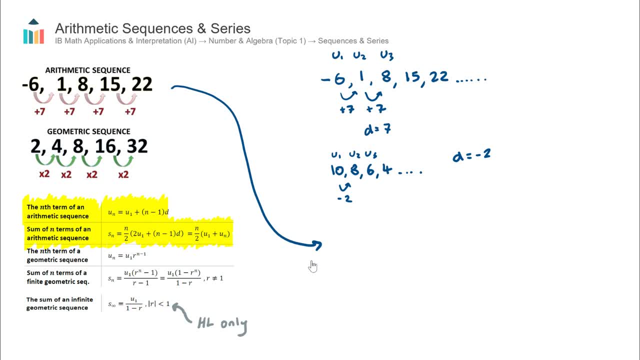 So what if we wanted to find the 15th term? Well, the correct notation is U15. In other words, I'm finding the 15th term. And that will be equal to, let's have a look at this formula here. It's the first term, which we know as negative 6, plus, we have brackets n take 1. n is the term number that we are looking for. 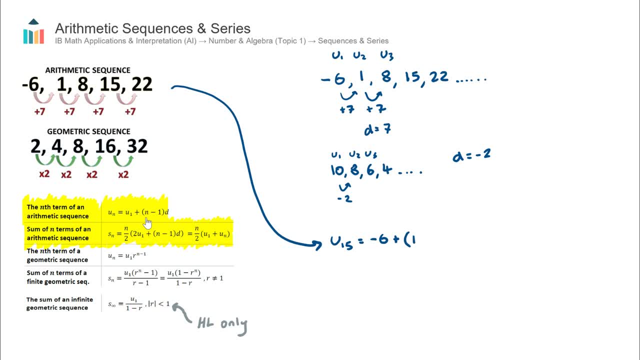 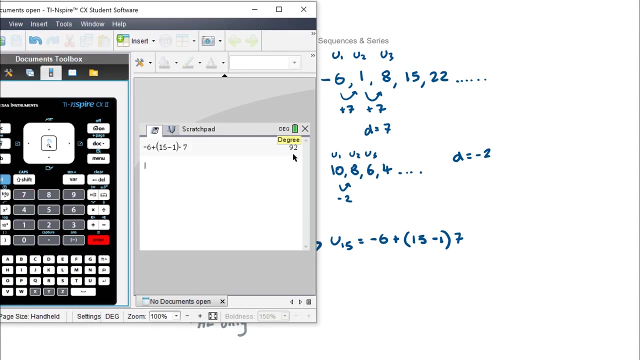 In our case, we're looking for the 15th term. So it's going to be 15. Subtract 1, multiplied by our common difference. Now we identified earlier that the common difference is 7. Now we can use our calculator from here to find out what the 15th term is. So I bring up my calculator. I did this just before this video. I hit Enter, and I get a 15th term value of 92. So U15 is equal to 92. 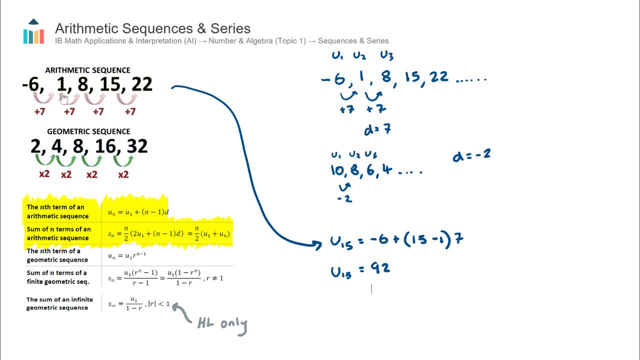 So if I was to keep progressing these numbers up, negative 6, 1, 8, et cetera, et cetera, up to the 15th number, that number would be 92. 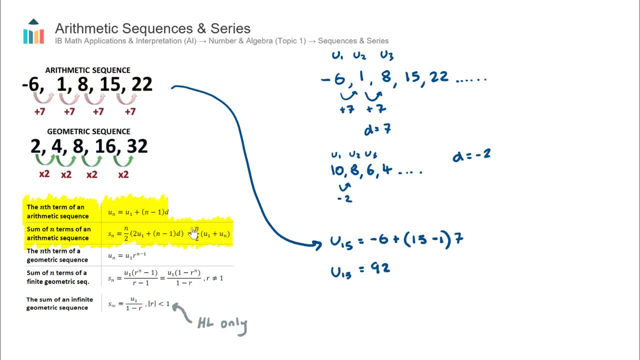 Now the second formula, and there's actually two here, we'll talk about both, is to not find the term number. It's to actually find the sum of a certain number of terms. And that's what a series is called. A series is summing up the terms in a sequence. So let's use this example again. 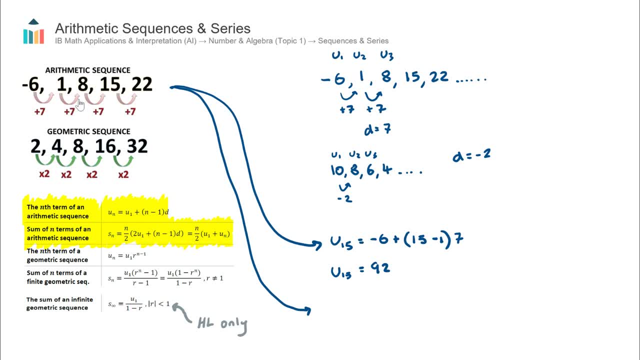 And let's say I was to ask you to find the sum of the first 10 terms in this sequence. So if I was to add up negative 6 plus 1 plus 8 plus 15 plus 22, find the first 10 terms and add them up. Well, if I was to do that by hand, that would take quite a long time because I would firstly need to find the 6th, 7th, 8th, 9th, 10th term and then add them all up. But fortunately, we have a formula here. I'm going to use the left-hand one, and then I'll explain the right-hand one after we find out what the answer is. Okay. 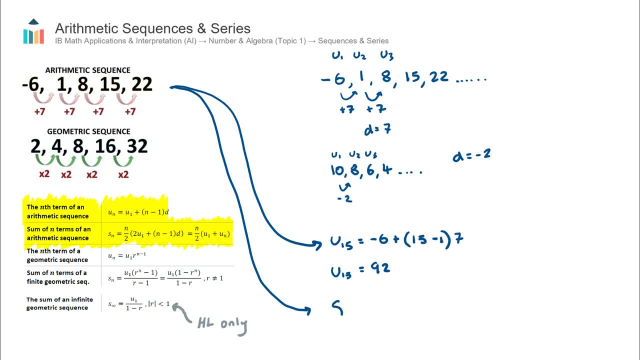 So the correct terminology, or sorry, notation, is the sum of the first 10 terms. And that is equal to, let's have a look at the formula. It is n over 2. Now we're looking to find the sum of the first 10 terms. So it's going to be 10 over 2 multiplied by 2 times the first term, which is negative 6, plus, again, n is 10. 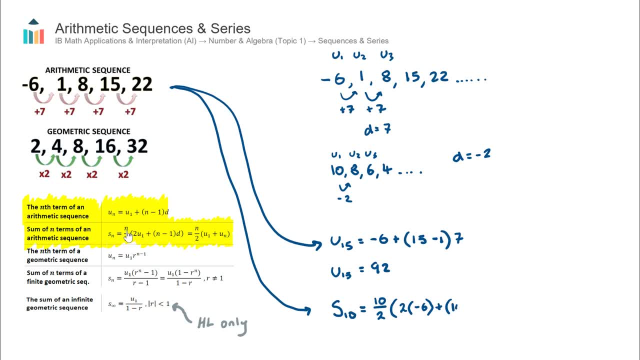 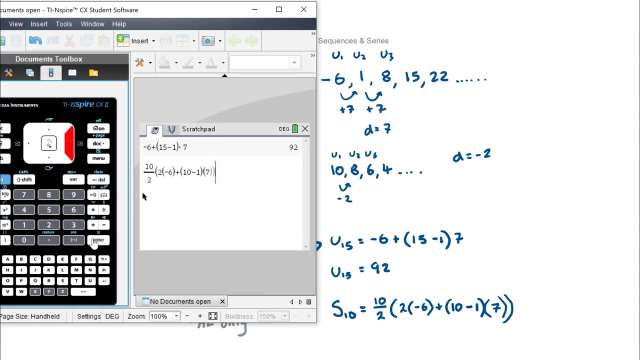 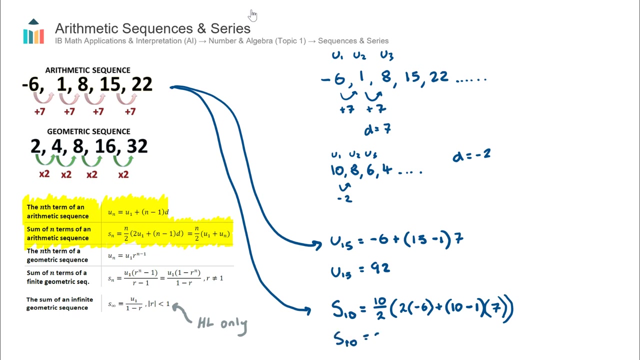 We're looking to find the sum of the first 10 terms. Take 1 multiplied by the common difference, which we know is 7. And again, we can use our calculator to find the result of this. And I just entered that there. And that is 255. So the sum of the first 10 terms, if I was to add them all up, would be 255. 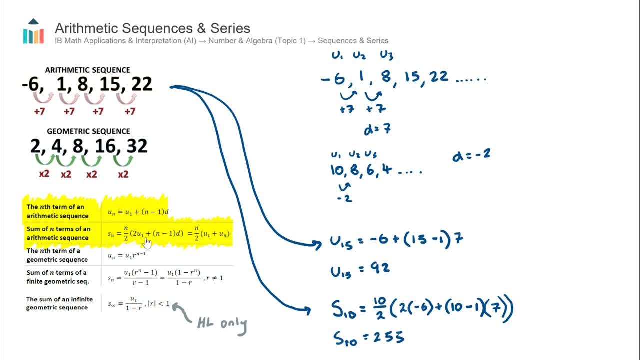 So we use the left-hand formula here to find the sum of the first 10 terms in this sequence. The right-hand formula, I don't use this all that much 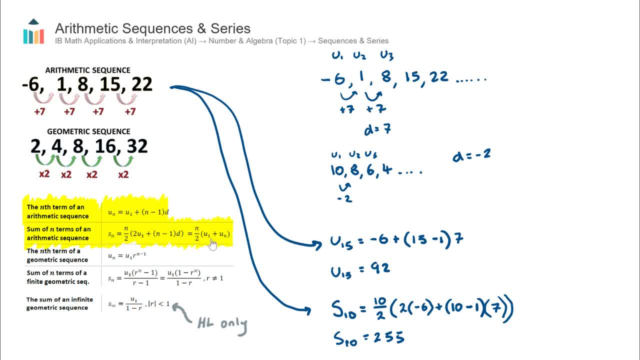 because it's pretty rare that you can use it. It comes up once every sort of 5 or 10 questions, maybe. 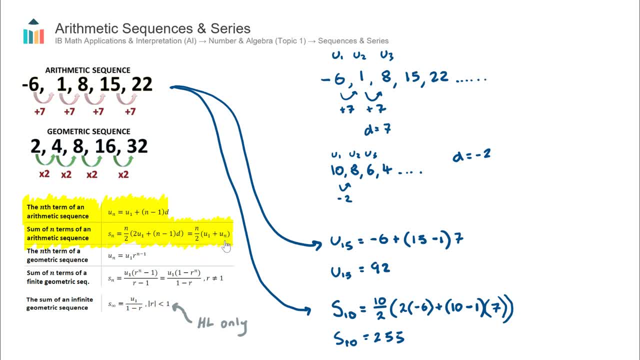 Now we can use this if we happen to know the final term. So in our case, in our sequence, we were finding the sum of the first 10 terms. 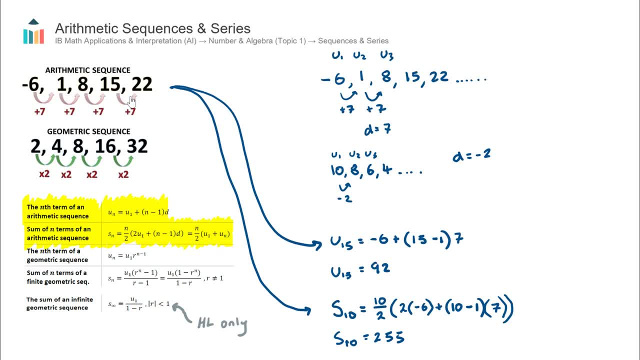 If I did know the 10th term value, which I didn't, but if I did, I could use this formula, 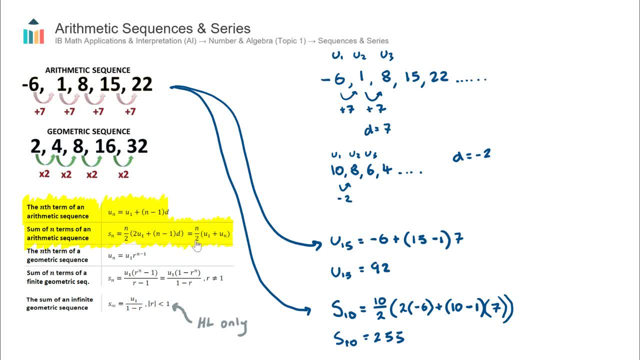 which is slightly easier to use. It would be 10 over 2 multiplied by the first term plus the 10th term.